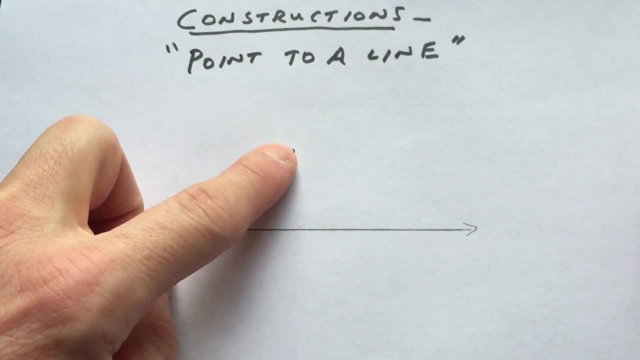 So when you measure the distance from a point to a line, you want to measure the shortest distance, the perpendicular distance. Otherwise, if you try to measure from a point to a line like this way or this way, or over this way, you know those are all going to be different. 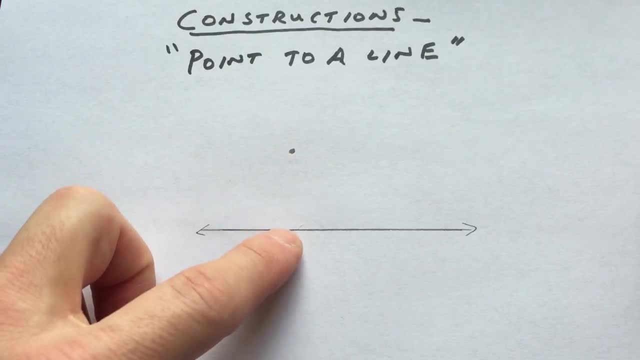 distances. There's only going to be one shortest distance from the point to the line, and that's going to be the perpendicular distance. So the way we're going to do this, this is very similar to when we found the perpendicular bisector. I showed you about that in one of 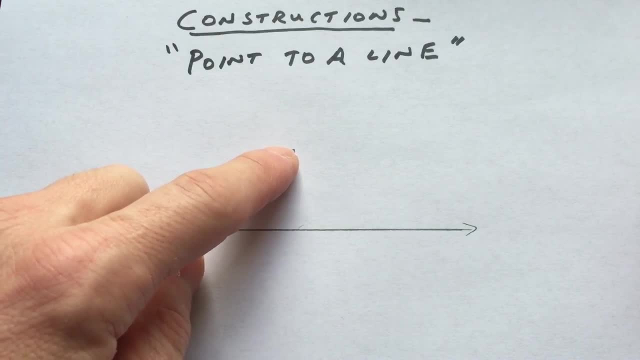 the previous videos. but what we did is, you know, we drew a perpendicular and we bisected the segment. We're going to do something similar here. We're going to find the perpendicular from the point to the line. So what I'm going to do is I'm just going to rotate this a little. 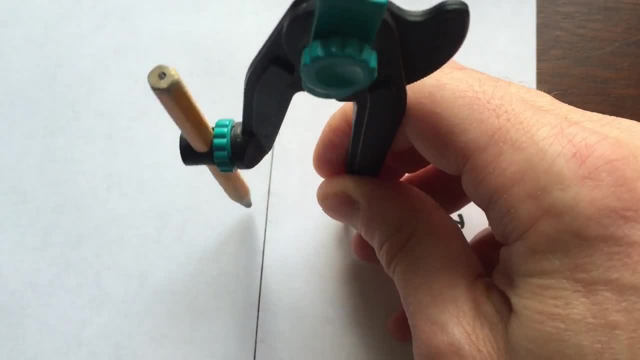 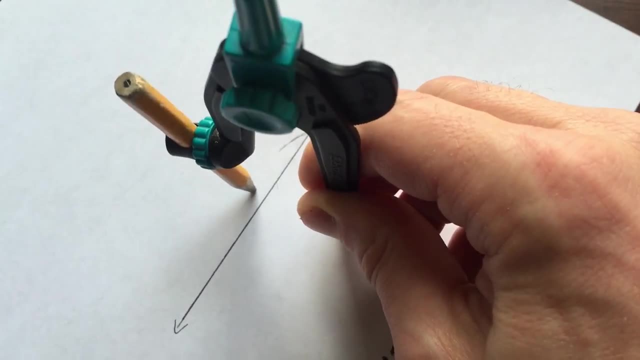 bit here and I'm going to draw. I'm going to open the compass, okay, and what I'm going to do is I'm going to draw two arcs, okay, and if you want, you can make this one continuous arc. okay, or you can pick it up and you can make it two separate arcs. So you can either. 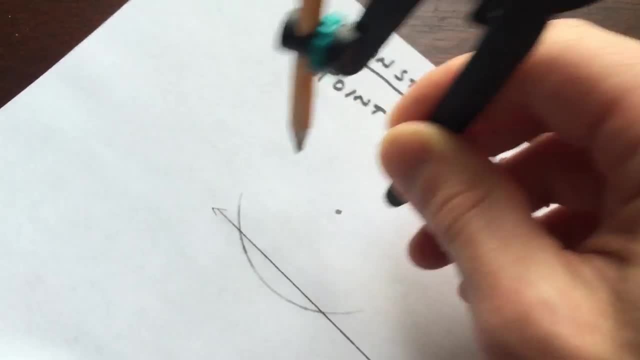 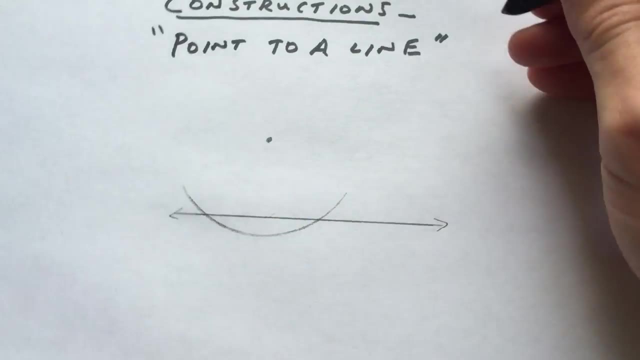 go like that, or you can just make it one continuous arc. Okay, so then, what I'm going to do is I'm going to use this point of intersection and this point of intersection to draw two more arcs, So I'm going to rotate the diagram a. 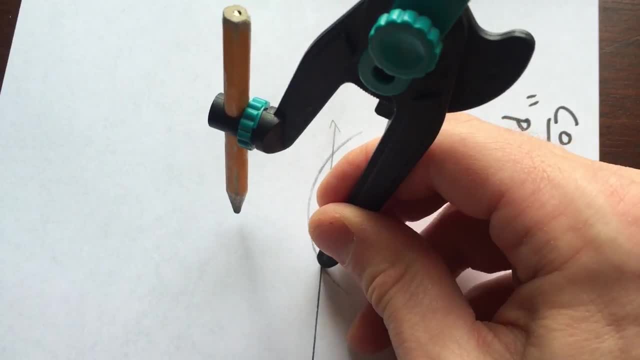 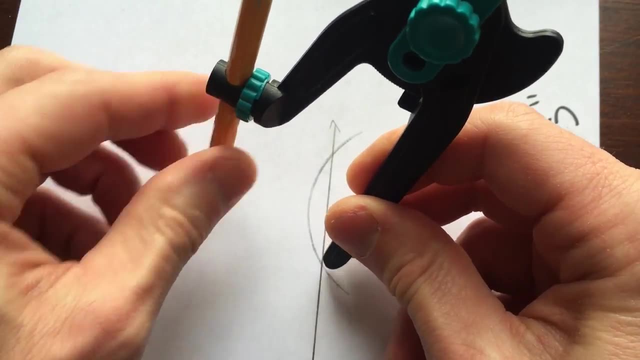 little bit here so you can see it and I'm going to use this point, and I'm going to use this point Now you can change how open the compass is at this point. I'm just going to open it up a little bit more, okay, and I'm going to make an arc like this. I'm going 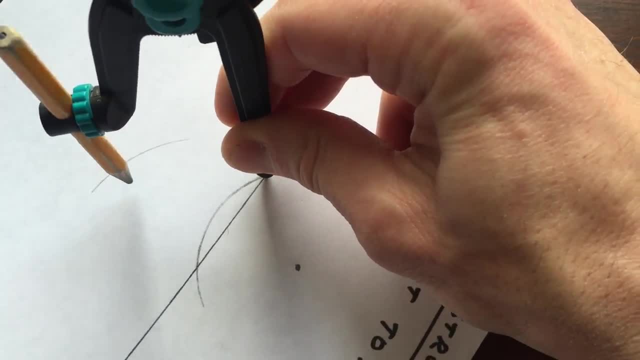 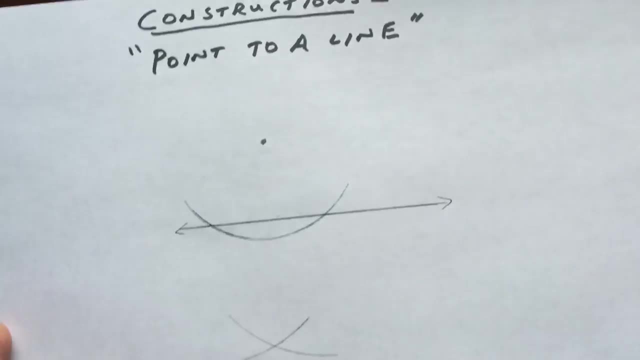 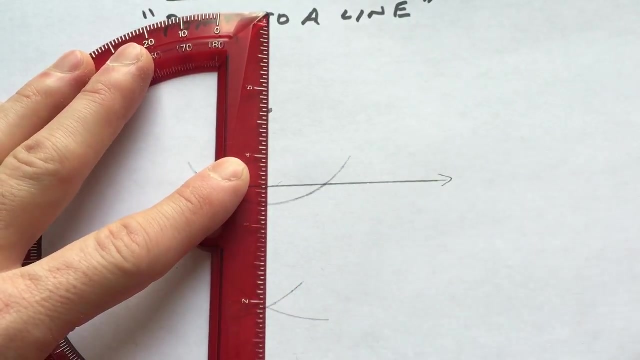 to go to the other point of intersection here, keeping that same setting on the compass, I'm going to make a second arc and then what we're going to do is we're going to draw a line that goes through this point and this point. So let's go ahead and do that, Okay. 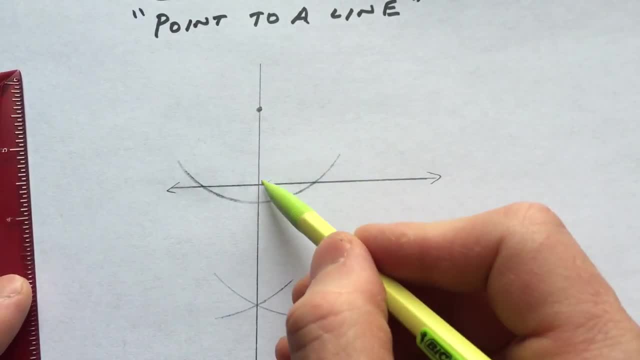 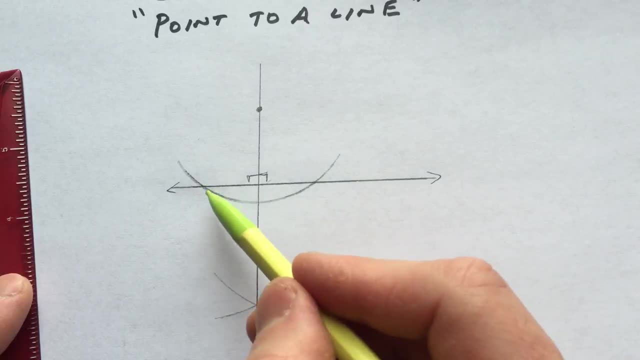 now you can see, all right, that this is perpendicular. It's a 90 degree angle, okay, and if you look, this is actually going to be the perpendicular bisector of this segment from here to here. So we're just drawing the perpendicular from this point to this line, but in actuality,